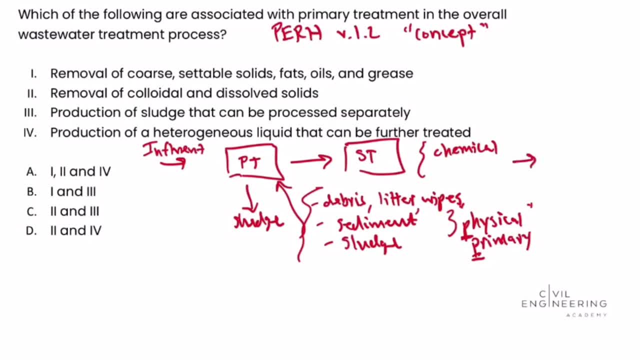 Right, And then it would go on further in the wastewater treatment process. So for the sake of time, we'll just focus on the primary treatment process. So let's look at the Roman numeral choices to determine the right answer to this problem. So 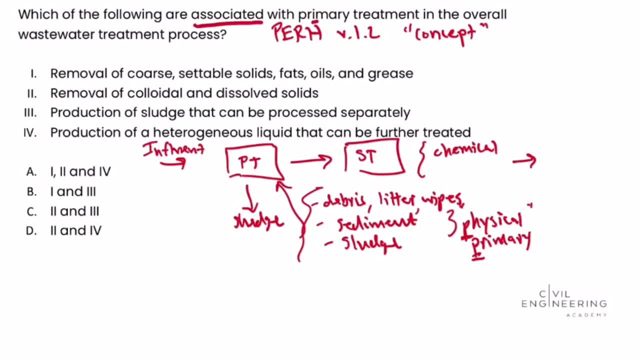 So which of the following is the right answer to this problem? So which of the following is the right answer to this problem? So those choices are associated with the primary treatment. So let's stay on task and look at these choices. So, Roman numeral 1. Removal of coarse settable solids, fats, oils and grease. 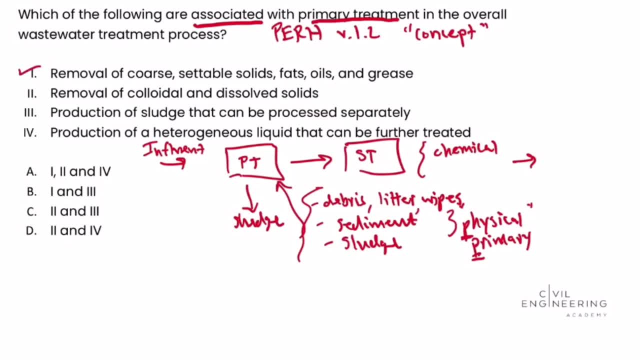 So yes, that is involved in primary treatment. Some of these physical things, like we said, the coarse particles, settable solids, fats, oils and greases, those will be eliminated in primary treatment Before that liquid goes on to secondary treatment. 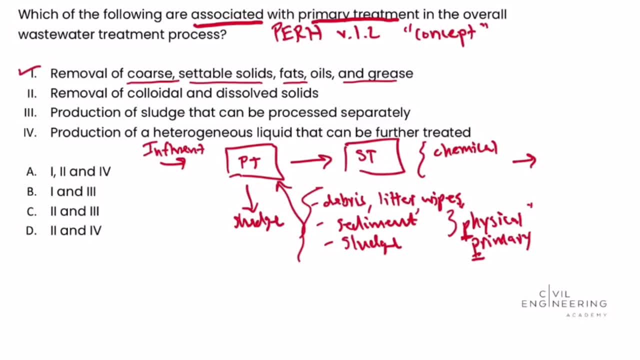 Removal of colloidal and dissolved solids. Well, dissolved solids and colloidal solids are within that wastewater influence stream coming in. They remain in it in primary treatment and continue on to secondary treatment untouched. These are handled in secondary treatment, not primary. So Roman, numeral 2: 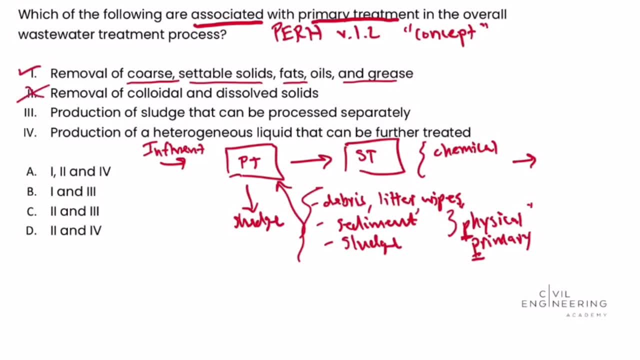 is not applicable. Roman numeral 3,: production of sludge that can be processed separately. So yes, in that primary treatment process, these items that we talked about that settle out, settle out into this sludge that's then handled separately. So yes, Roman numeral 3 applies to. 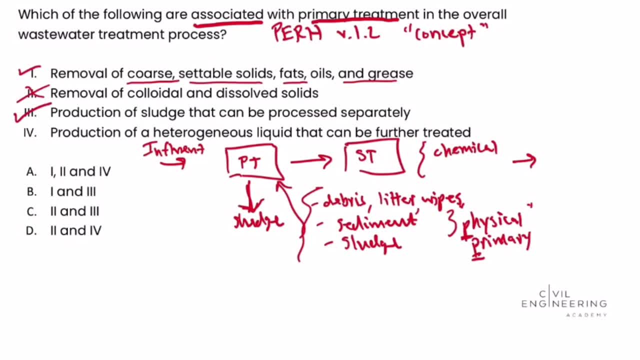 primary treatment. Roman numeral 4,: production of a heterogeneous liquid that can be further treated. Well, we said yes. the goal of primary treatment is to produce a liquid that could go on to secondary treatment, but it's a homogenous liquid that's produced. 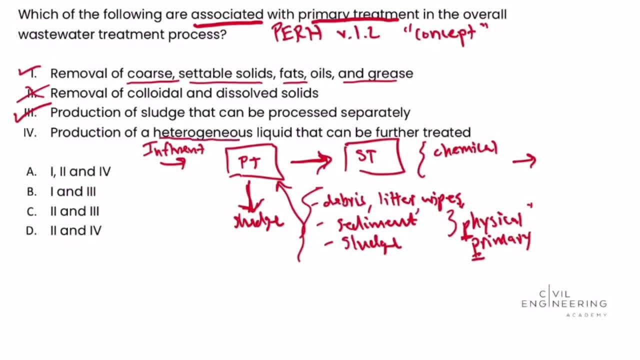 Roman numeral choice 4 says heterogeneous. We want a homogenous liquid being produced for that statement to be true. So Roman numeral 4 is not correct. We need to be careful and read it carefully. the heterogeneous versus homogenous. That could throw us off if we're not careful. 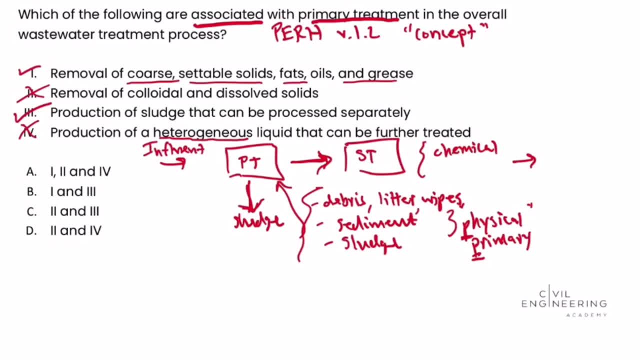 So that leaves us with Roman numeral 1 and 3.. And looking at the answer choices, that is answer choice B, And we've successfully solved this problem. So I hope you enjoyed this video. If you did, please give it a thumbs up and subscribe to our